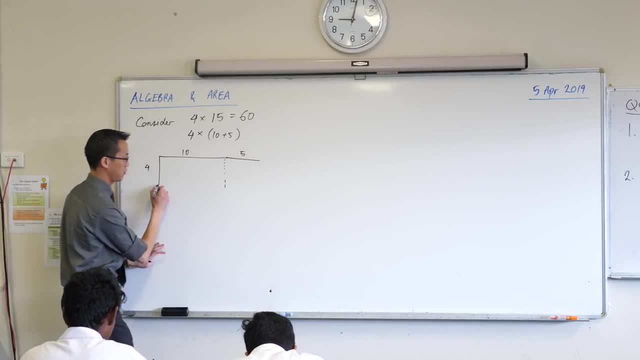 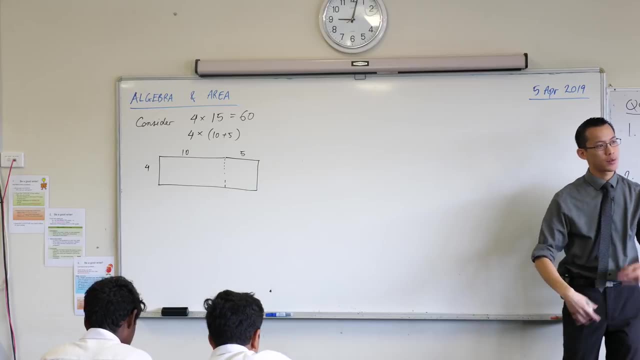 So what I'm going to form here is a couple of rectangles. It looks like. so Okay, Now let's have a look at this together. I mean, you already kind of know the answer, but I want to show you why the answer is what it is. Where'd my orange go? Oh, where did my orange go? Here, it is Okay. 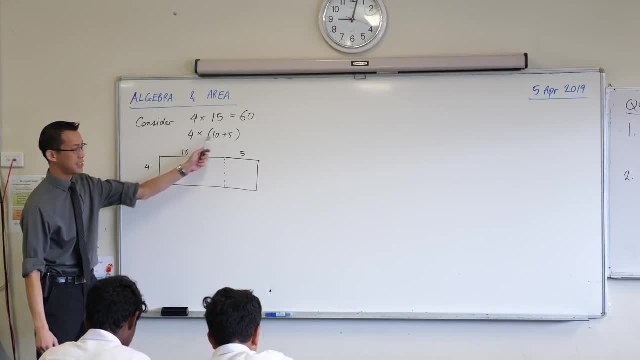 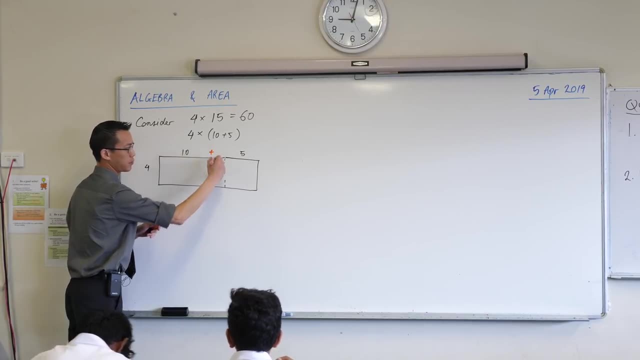 Okay, 4 times 10 plus 5, I can say it's kind of like the area of this rectangle 4 times 10 plus 5,, okay, And so the whole rectangle kind of is in two pieces. Can anyone tell me this left-hand piece, what's the area of this side? It's going to be 40, right, 4 times 10, it's just length times breadth, isn't it 40.. 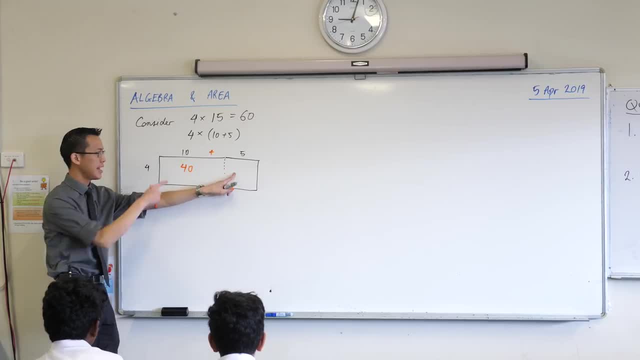 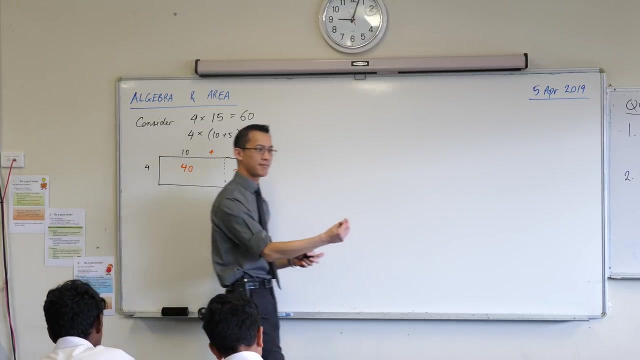 And then you've got this other smaller rectangle over here. It's not 4 times 10,, it's 4 times 5, which gives you an answer of 20. Which agrees with what we found before. right, The total area 40 plus 20 gives you that 60,. okay, Now, this is nice with numbers, but we can extend it to algebra, because these pronumerals and things we're dealing with, they just kind of stand in the place of numbers. 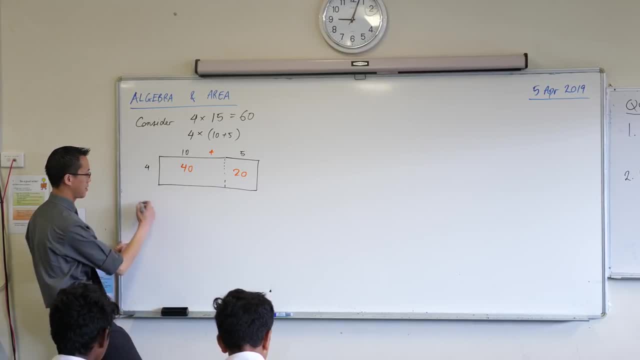 For example, if we said we had 4a minus 3, I'm going to change it. Let's consider 4 with an a plus 3 instead. It's a little bit easier to conceive of if everything's addition. Can you draw for me the same rectangle, but just we're going to label it. 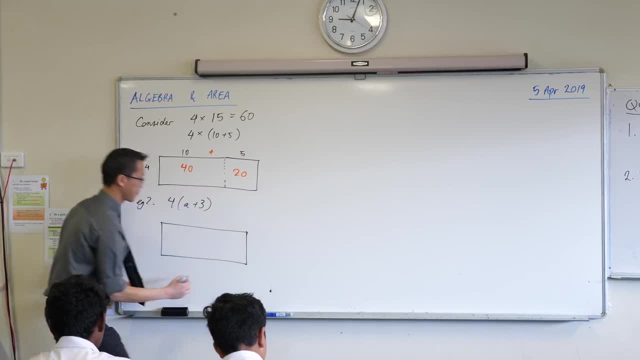 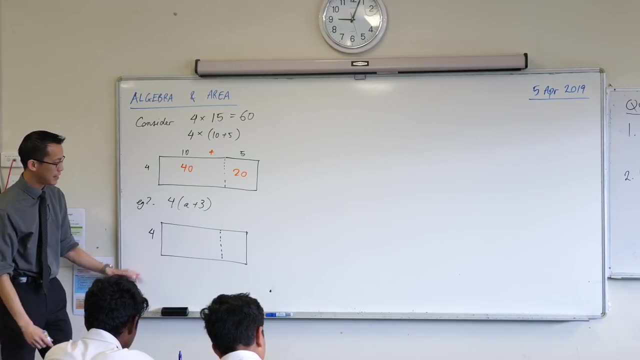 Differently. Same rectangle, but this time I'm going to put some different numbers on it. I've got a 4 over here, just like before, but instead of 10 and 5, which is what I had inside the bracket before, what shall I label on my tops here? 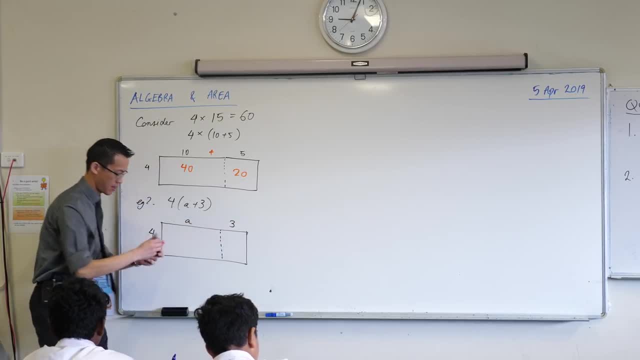 a and 3.. a and 3.. Now, for anyone who looked at those ones before, the expansion is still a bit funny and confusing. right, Can you see how this gives us the two terms? It's why I'm distributing the 4 to the a and the 3.. 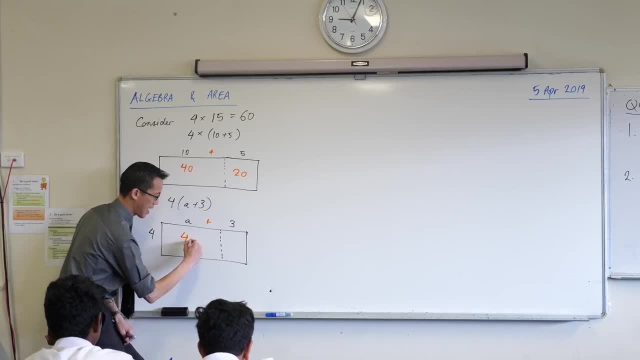 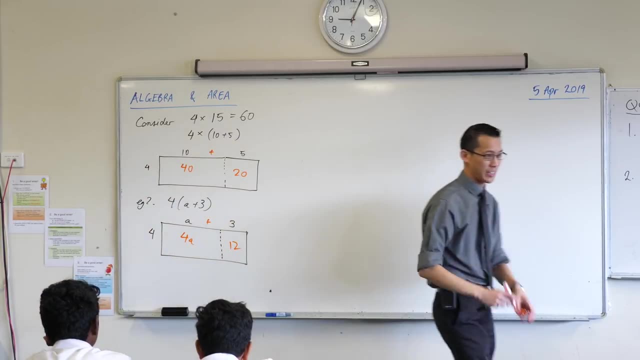 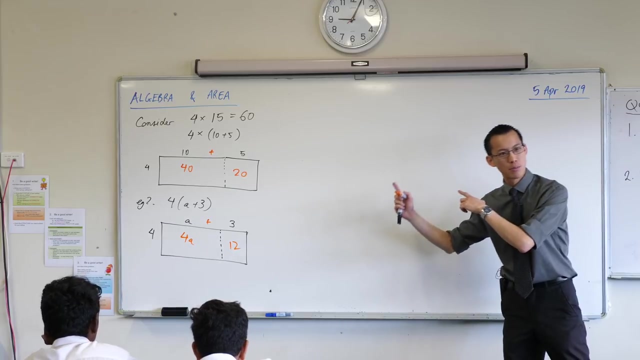 What's the area of this part here? It's 4a, very good, And then this leftover part: it's 4 times 3, which gives you 12.. Thank you, Barabi. Okay, now this is another thing. We know how to do this already. You're like, I didn't need to draw a diagram in order to know the answer to these, but I can use this diagram to help me try out some more challenging things. 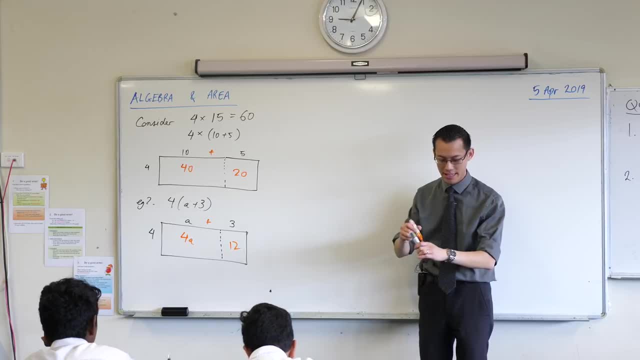 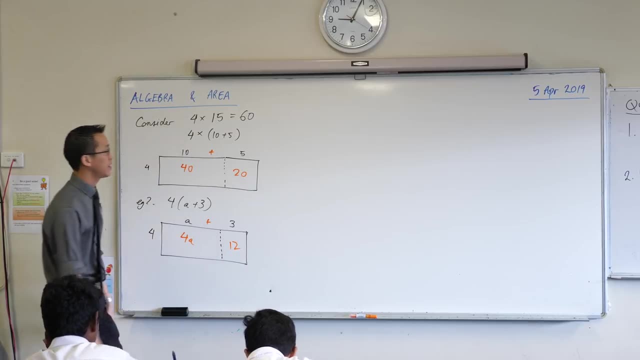 Okay, now see how we've got some numbers here, and then we've got some algebra. In the same way, I want us to extend our numbers. I want it to be two-digit, okay. So see how we've got 4 times 15 here. 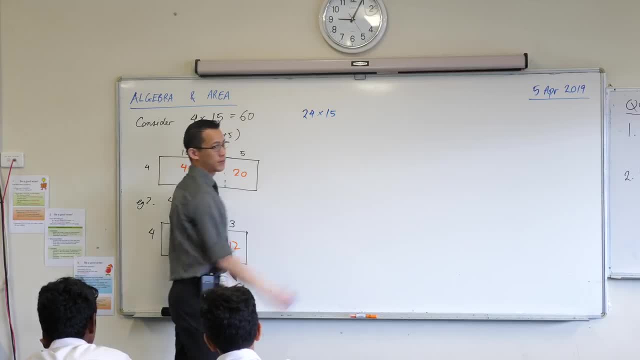 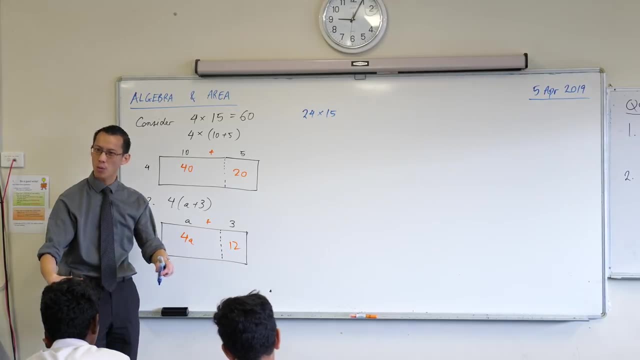 I'm now going to try out 24 times 15.. Now you all did 4 times 15, just without thinking right 24 times 15, I think you could probably work out with some time, but it certainly doesn't jump out at me what that answer is immediately. 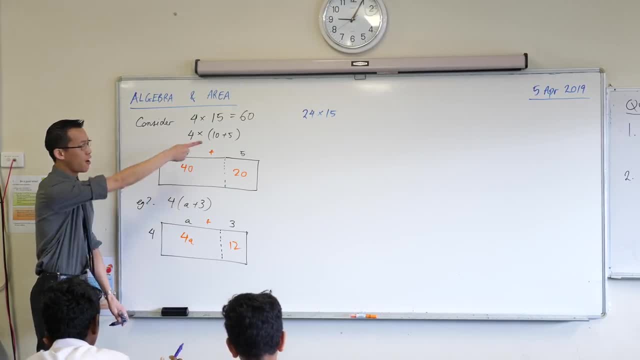 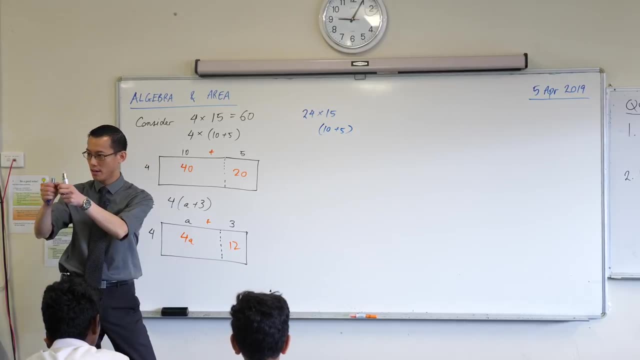 But I can use that same model to help me out here. You know how I break apart the 15 into 10 and 5?? I can also break apart the 24, right, It's well, how am I going to break it out? 20 and 4, my 10s and my units. 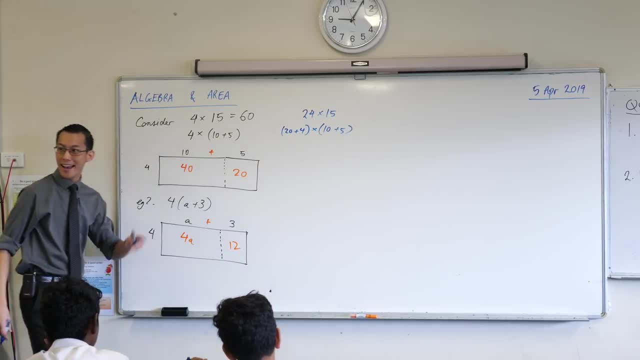 20 plus 4, like. so, okay, Now I can use this. maybe you're like: I just worked out the answer, right? Okay, I'm going to confirm whether the answer is what it is by drawing up another area model, another rectangle for myself. okay, This one's going to be a little bit taller Now. 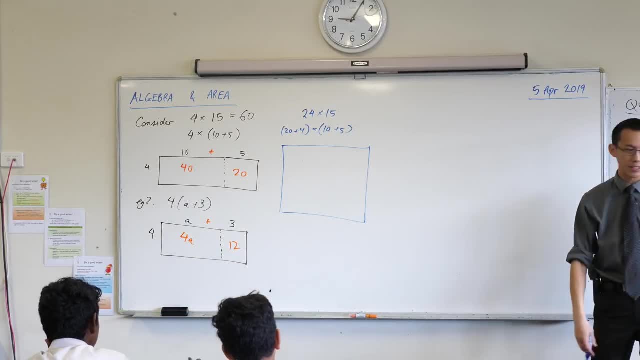 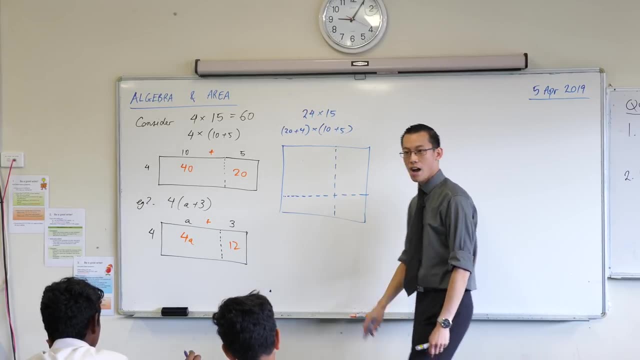 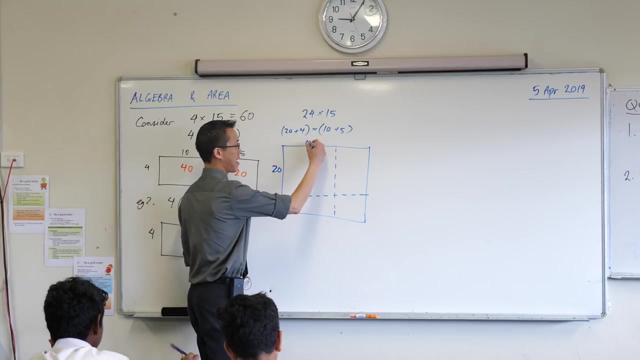 so far we've been trying to make it so that the scale is reasonable. it's going to start to get a bit harder here, but I'm going to draw across like: so I've broken up my rectangle into more pieces because I've got 20 and 4, then I've got 10 and 5.. Is this ringing bells for you? You're 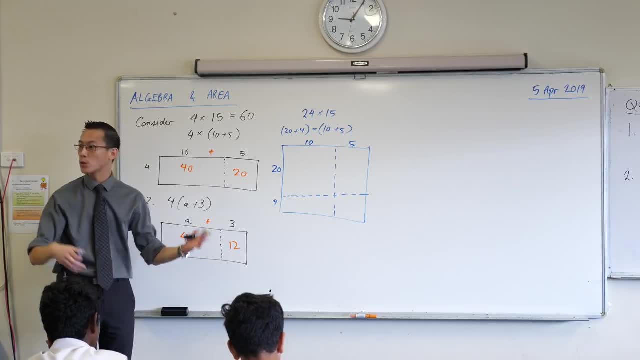 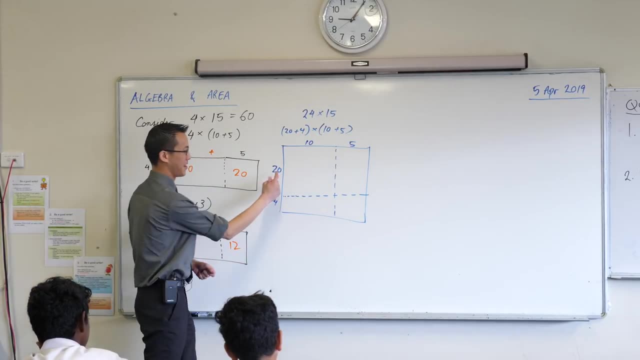 like I remember seeing this, I can work out each of those rectangles individually, which is much easier to do than doing the whole thing. 24, lots of 15 together, So one at a time, 20 times 10, what's this biggest rectangle here? 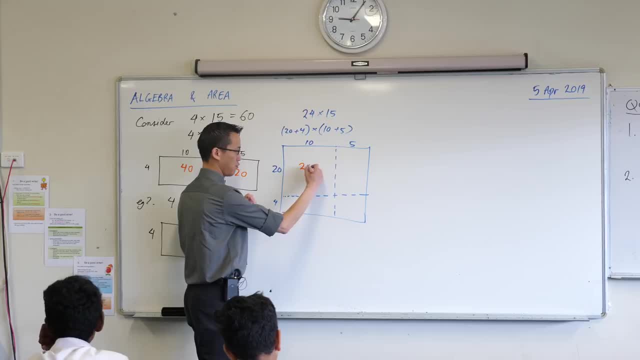 200,, 200.. How about 20, there's 20 again times 5? It's going to be 100, and then I've done those two. so now I'll do the bottom two, which are actually I kind of already did these before. 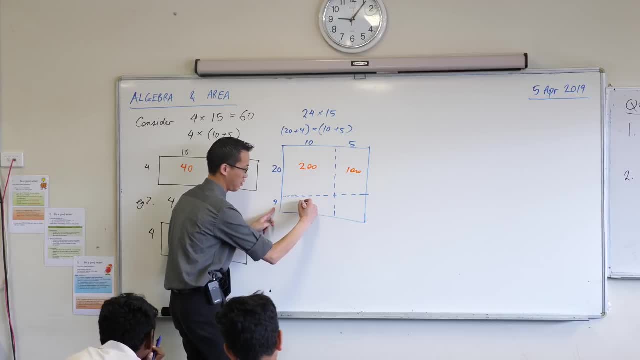 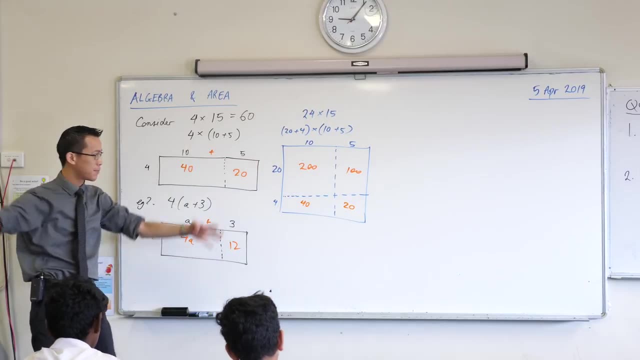 I'm cheating by using easy numbers. This is still 4 times 10,, so it's still 40, and this is still 4 times 5,, so that's still 20.. And so the total shape is going to be 1,, 2,, 3, 4, all added. 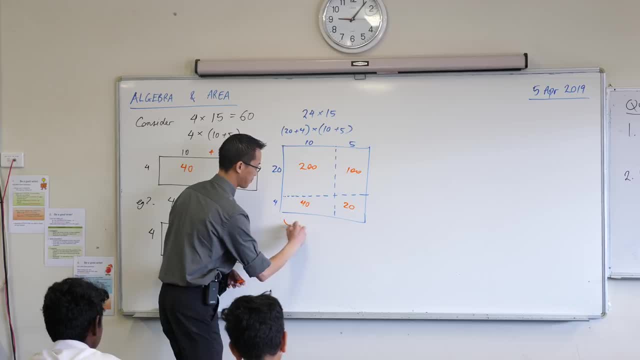 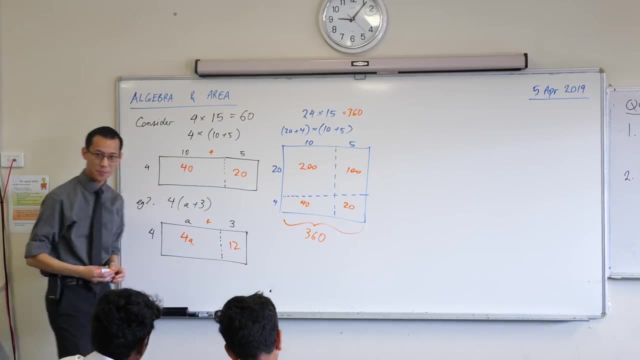 together. Can someone tell me 360.. 360, very good. So that's what 24 times 15 is equal to. Now I want you to think about what that might look like for something like this if it had not just 4, lots of a plus 3, here's where. 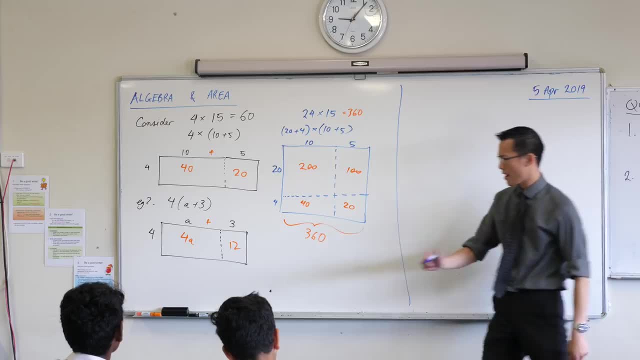 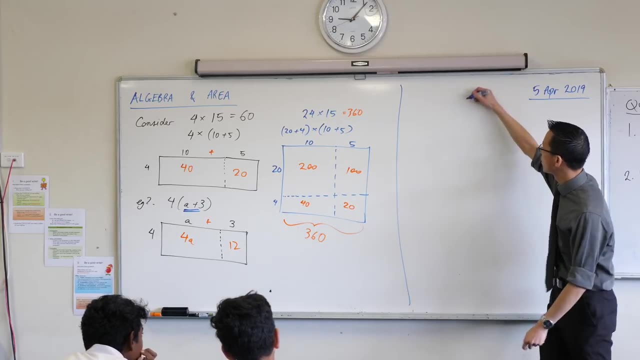 we're going. What if I had see that thing on the right-hand side, this guy here? It's got two bits to it, two terms. so we call it. we give it a special name. it's called a binomial. 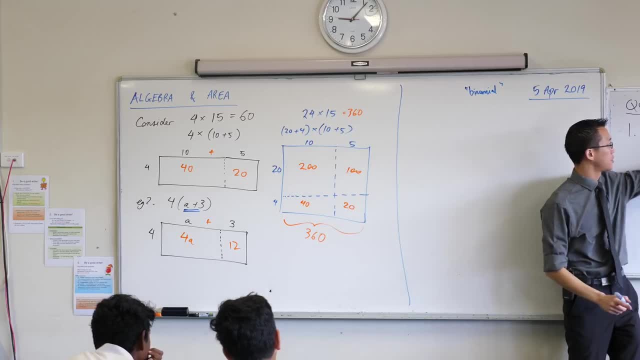 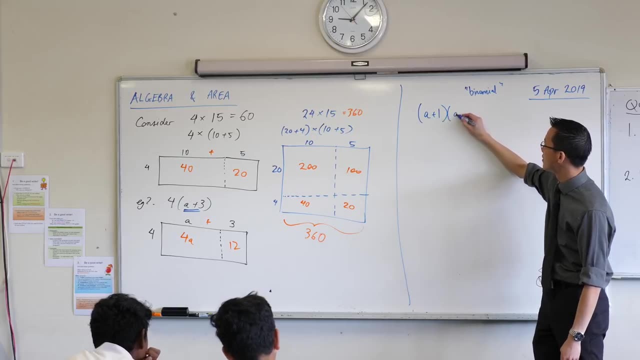 You've seen, by already just means two, and nomial means two terms. okay, So we're going to try this: a plus 1, a plus 3.. Now, this is new and this is why we spent so much time developing this to. 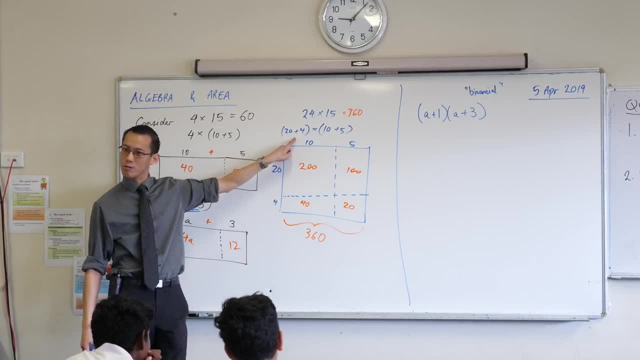 make sure we know what's going on. This is just like what we did here, right? There's a binomial here, two terms, binomial here, two terms, and I'm going to multiply this out. so can you draw a nice? 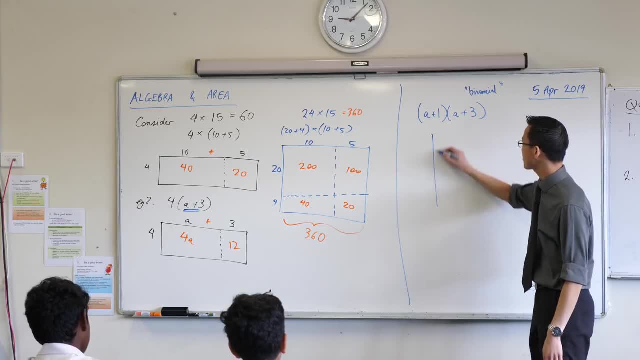 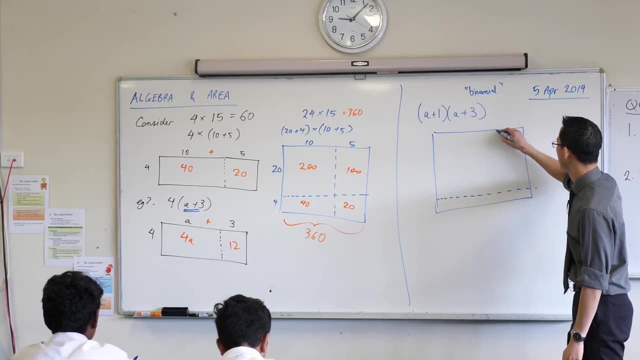 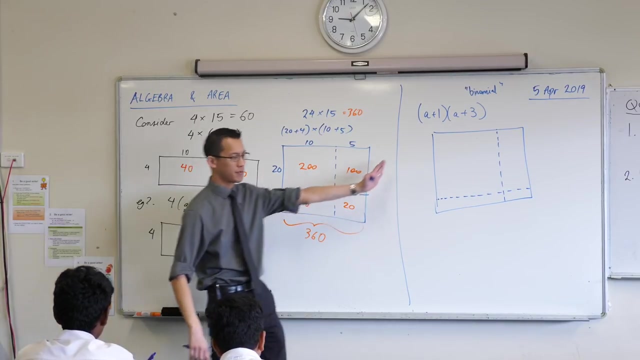 big rectangle for me and we're going to work out all of the pieces. Hmm, Okay, Now it actually doesn't matter which one you make which, but on this vertical length over here, I'm going to make that refer to this guy on the left-hand side. okay, So I've got. 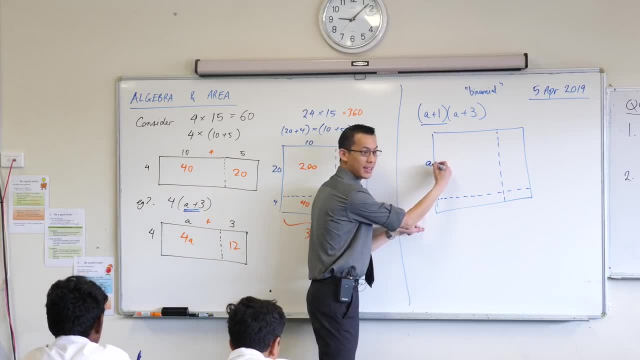 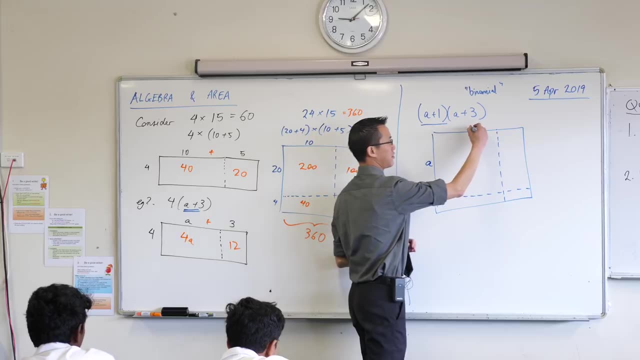 two lengths here, right, One of them is going to be a and the other one's going to be 1, so this height here is a plus 1, following so far The width, same deal: a, and then there's a 3, so the whole width is a plus 3.. 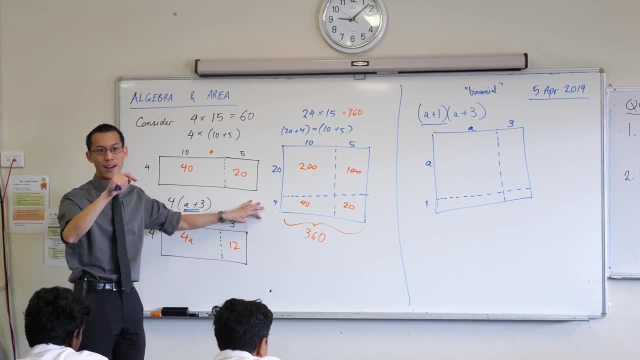 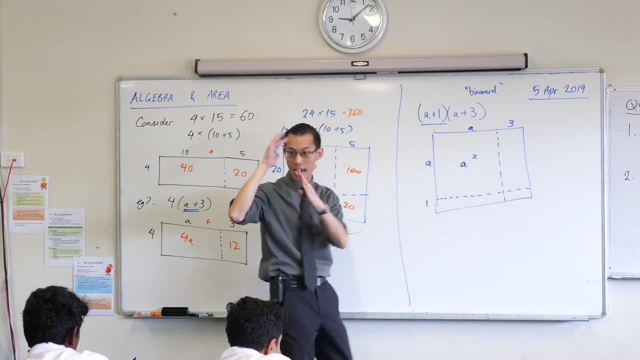 And now, just like we did with the numbers, we can think about each rectangle individually. Roshan, can you tell me what this rectangle here is going to be Very good, In fact. it's not just a rectangle, it's a square, because it's a by a. 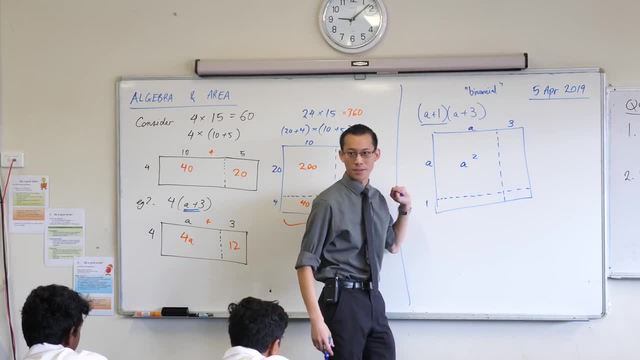 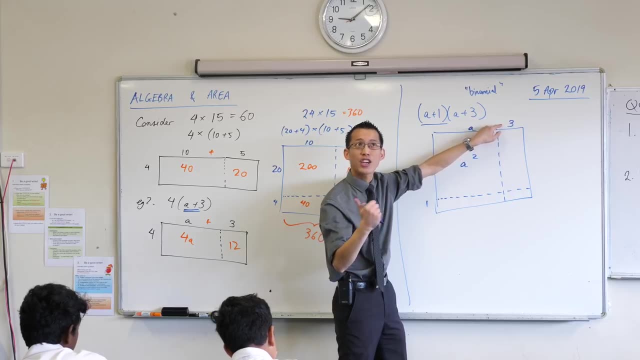 Anva, can you tell me what this rectangle over here is? the thin one, thin, tall one? Okay, now let's have a look carefully. You've got a height of a right And I'm going to use that 3, but a cubed is something else, isn't it? 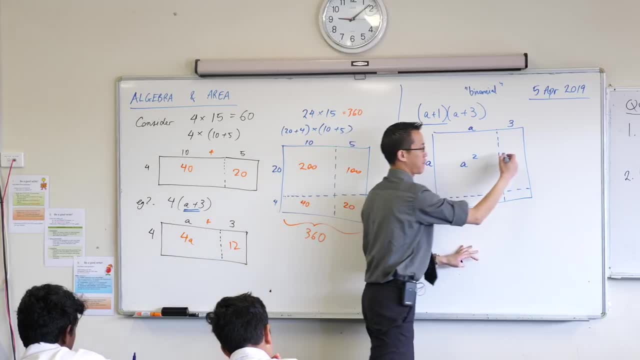 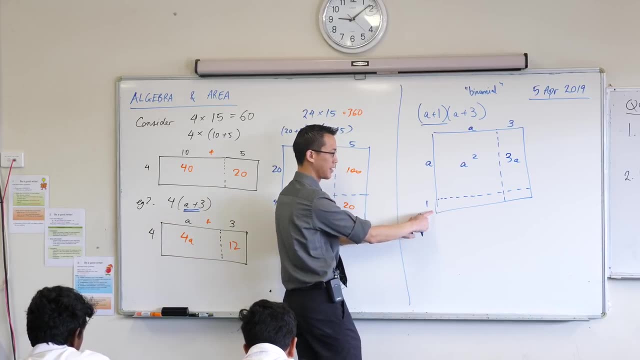 Yeah, it's going to be 3 multiplied by a, so 3a is exactly right, okay. How about Roshan? can you tell me what this lower wide rectangle is? Yeah, a is just going to be the one lot of a, so there's an a there. 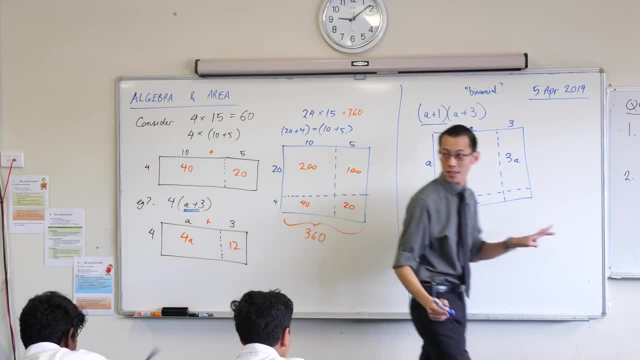 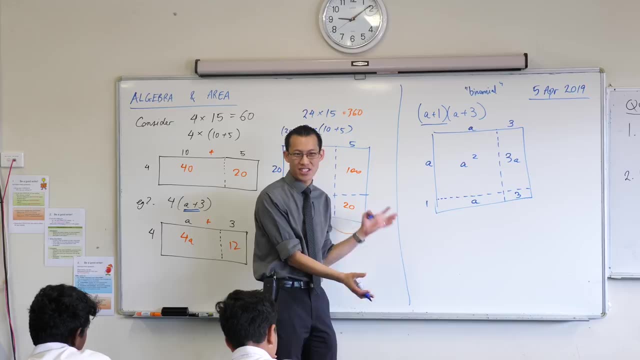 And then I've got my final little one in the corner. e-naught, can you tell me what that one is? 3,- very good. Now we got 360 by adding up all four of these numbers Here. I'm going to do the same thing, but there's just some algebra there, right? 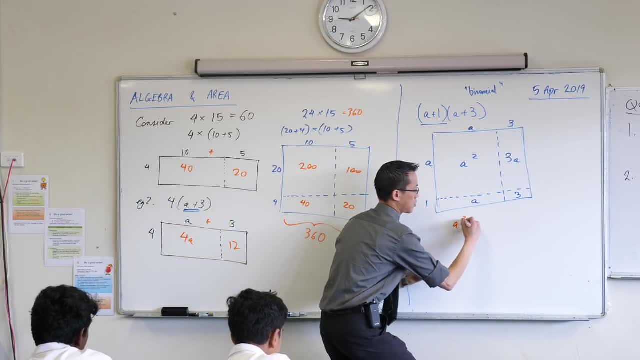 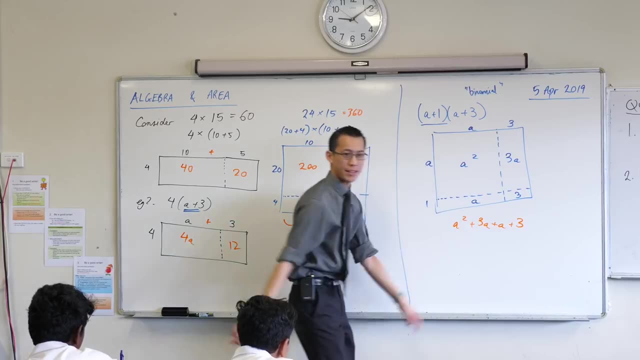 So, whoops, Here we go a squared. there's that one plus 3a. there's that one plus a plus 3.. That's the whole shape. Can we write this any simpler? We can right. What are we going to do? 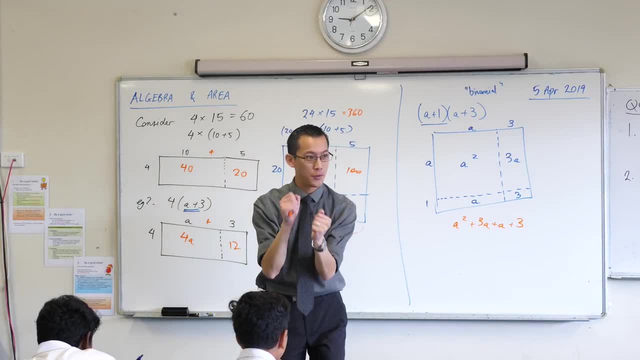 Ah, now, now let's think about this. We've seen this a cubed come up a few times, right? Can someone tell me what does a? it's an abbreviation, right? What's a cubed? an abbreviation of Roshan. 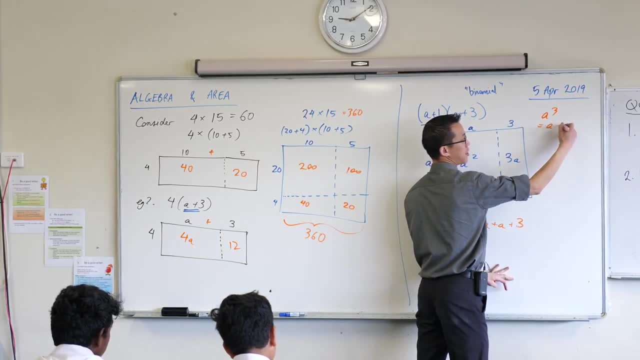 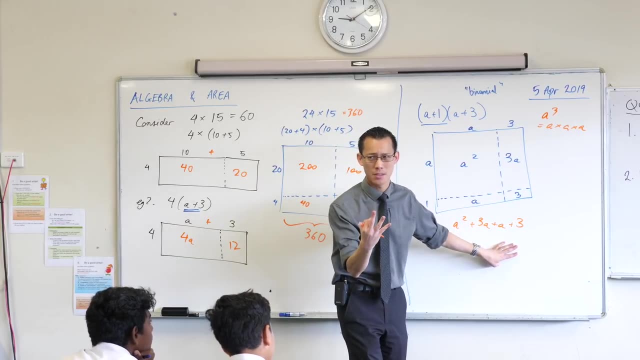 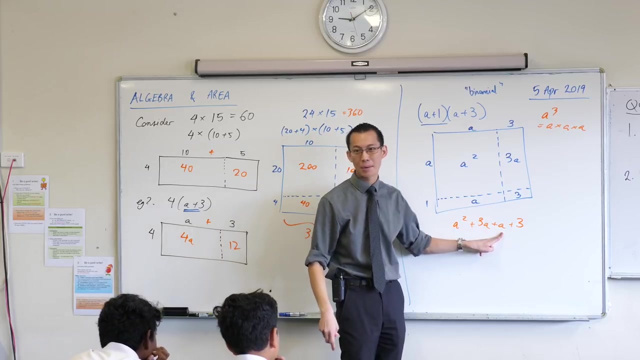 Multiplication. A cubed is about multiplication: a times a times a. Is there any way here that we see a being multiplied by itself three times? Hmm, I see a multiplied by itself twice. I see a 3 times a and just a single a, but I never see a times a times a. so I'm going to leave that a cubed out of it, okay. 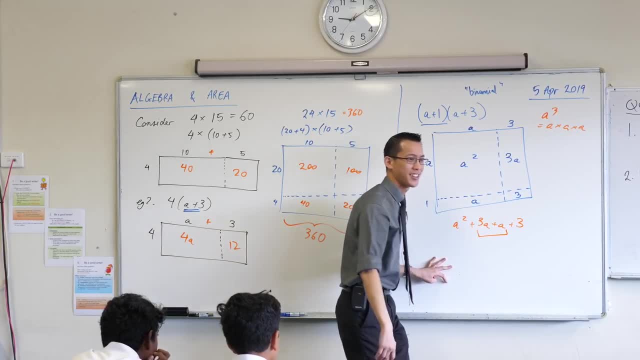 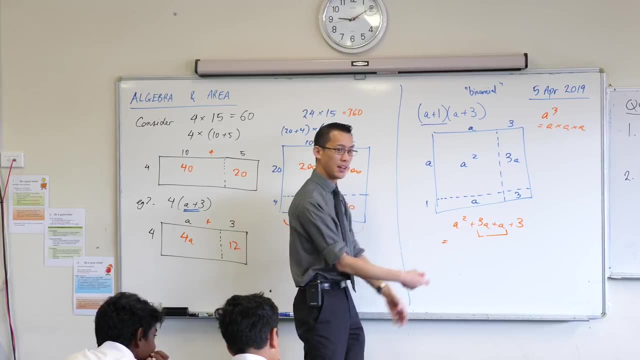 There is something else I can do with these two in the middle, though. what would you like me to do, Louise 4a? Yeah, this is called. does anyone remember this? It's called collecting, like terms, These a's in the middle. there's 3 over here, 1 over there, so that gives me 4 in total. 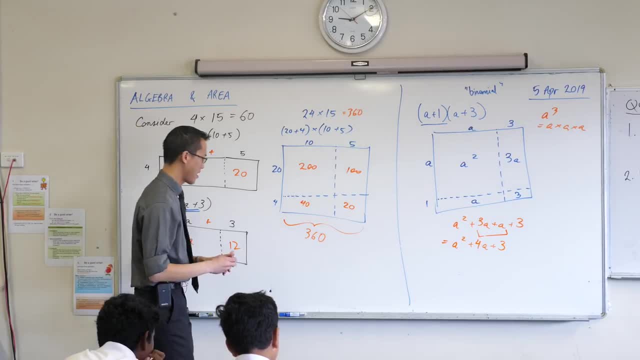 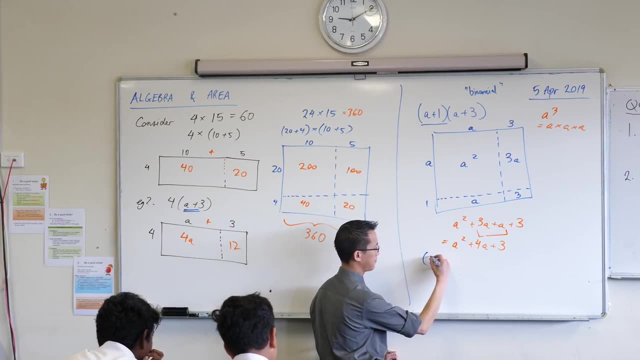 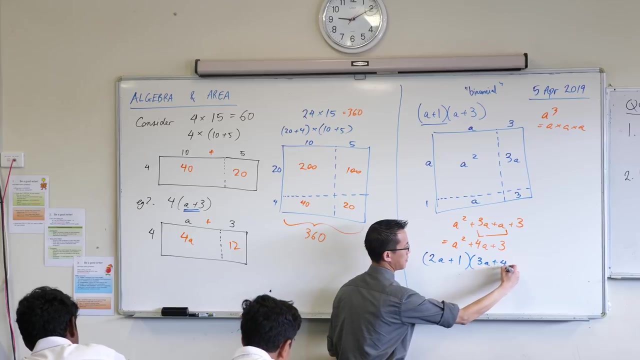 Does this make sense? Okay, let me try another one for you. Draw the diagram for this: Instead of a plus 1, a plus 3, I'd like you to try one that looks like this: Now, one of the weird things about this- unlike with our numbers- is that you know 20.. 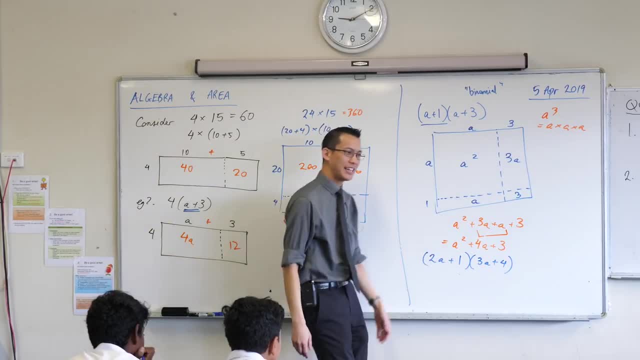 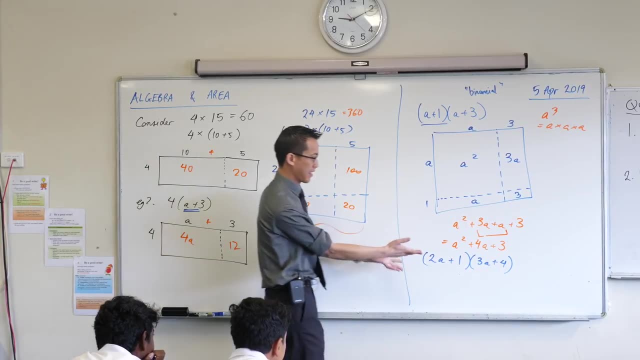 20 is going to be roughly that much longer than 4, but with a you're like I don't know what a is. a could be anything, so you can draw that to be a different length. it doesn't really matter all that much, just try and make it so it doesn't look too weird and out of proportion. 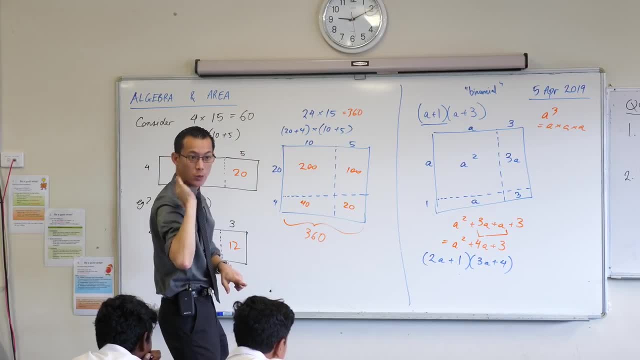 I'm going to give you a minute to try and draw up that rectangle. think about what that vertical length will be, what the horizontal length will be, and then we'll have a look at the solution together. I'll give you about 30 seconds.